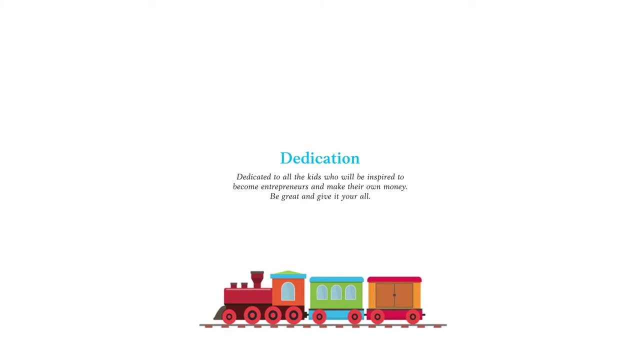 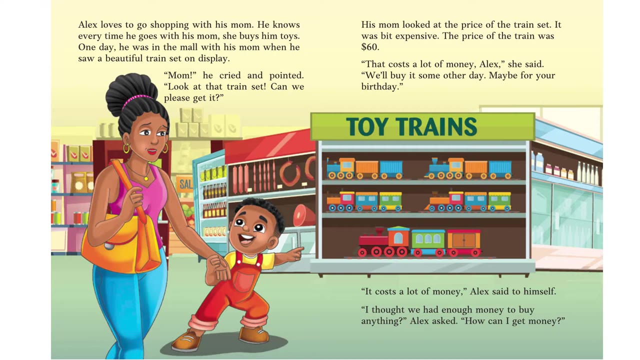 inspired to become entrepreneurs and make their own money. Be great and give it your all. Alex loves to go shopping with his mom. He knows every time he goes with his mom she buys him toys. One day he was in the mall with his mom when he saw a beautiful train set. 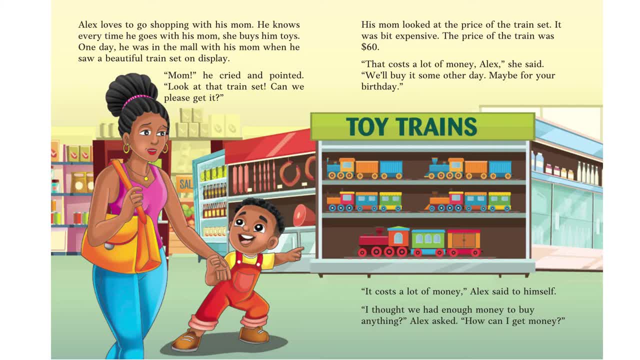 on display, Mom. he cried and pointed: look at that train set, Can we please get it? His mom looked at the price of the train set. It was a bit expensive. The price of the train was $60.. That costs a lot of money, Alex. she said We'll buy it some other. 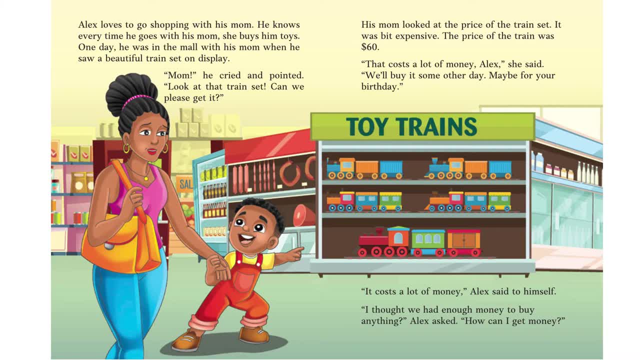 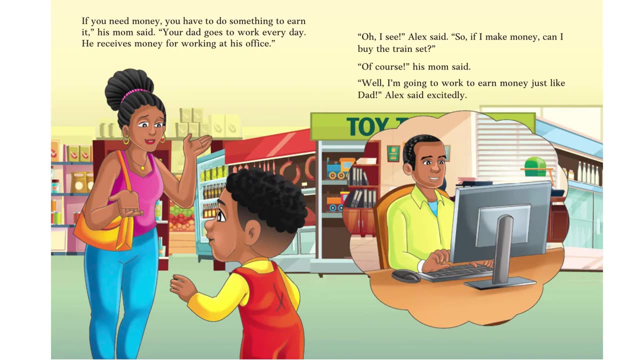 day, maybe for your birthday. It costs a lot of money. Alex said to himself. I thought we had a lot of money. Alex asked: how can I get money? If you need money, you have to do something to earn it. his mom said: Your dad goes to work every day. He receives money for working at his office. 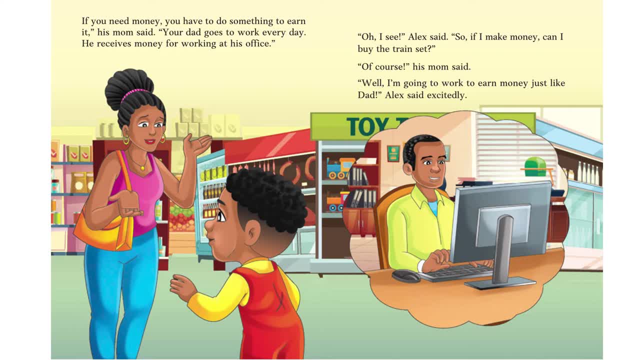 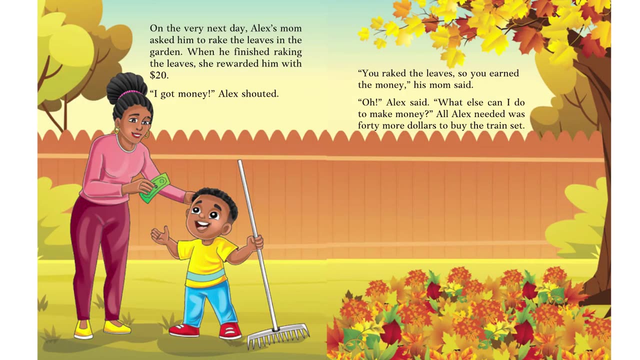 Oh, I see. Alex said: So if I make money, can I buy the train set? Of course, his mom said: Well, I'm going to work to earn money, just like dad Alex said excitedly. On the very next day, Alex's mom asked him to rake the leaves. 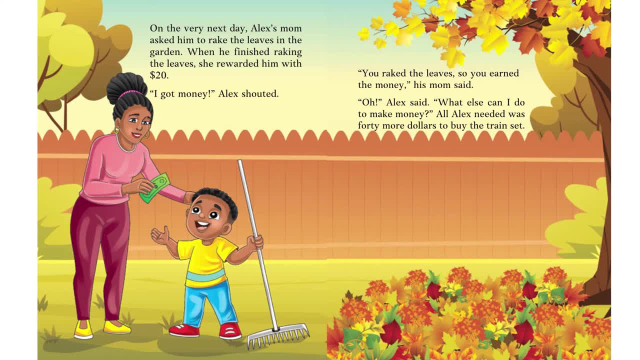 in the garden. When he finished raking the leaves, she rewarded him with $20.. I got money. Alex shouted: You rake the leaves so you earn the money. his mom said: Oh. Alex said what else can I do to make money? Alex said I don't know. I don't know how to make money. I don't. 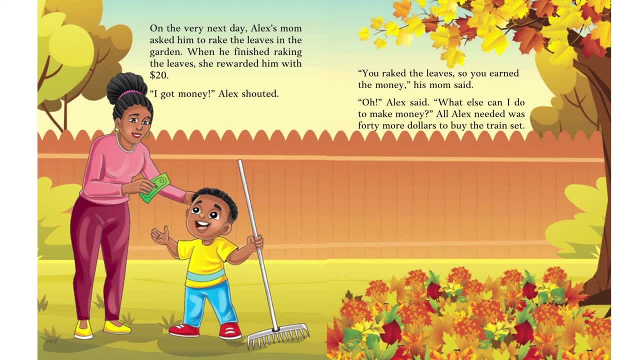 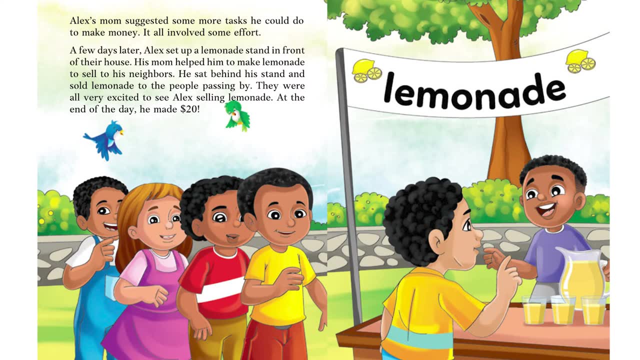 know how to make money. All Alex needed was $40 more to buy the train set. Alex's mom suggested some more tasks he could do to make money. It all involved some effort. A few days later, Alex set up a lemonade stand in front of their house.